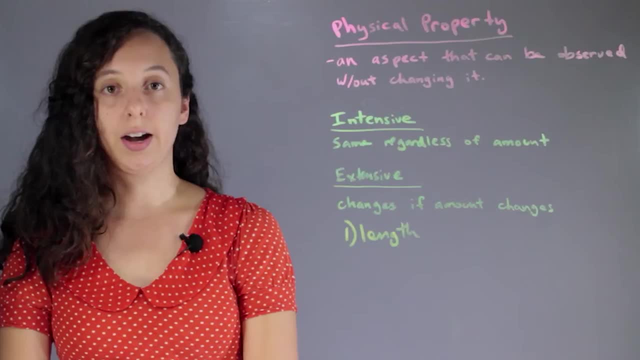 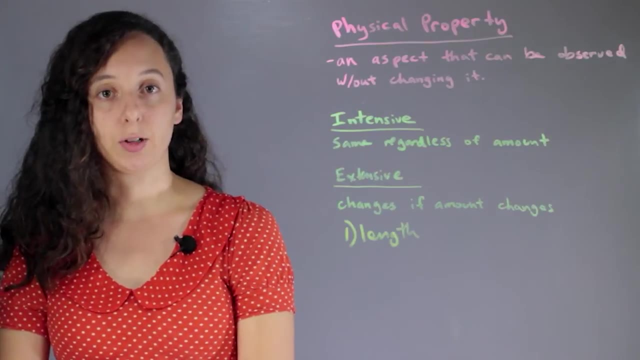 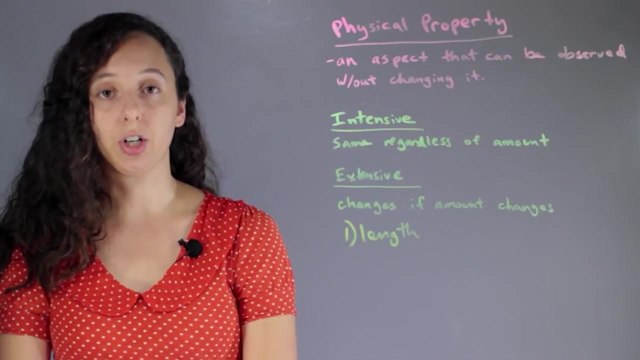 need to break anything or change anything if you just want to measure the length Physical property, Now the alternative is a chemical property, which is something that can only be observed by changing the actual chemical structure. So, for instance, if you light, 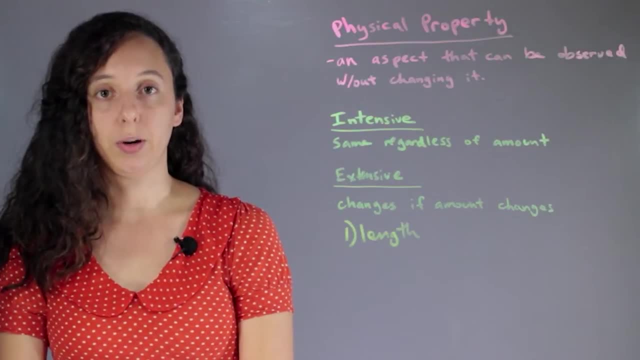 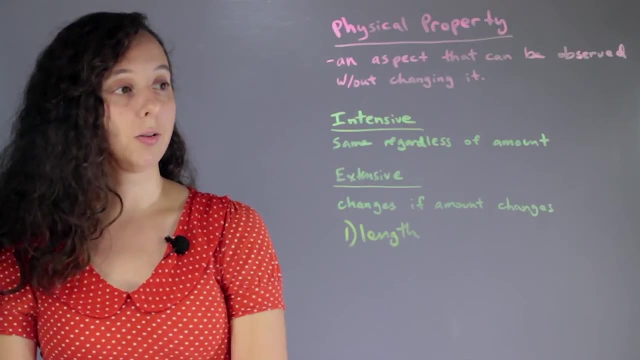 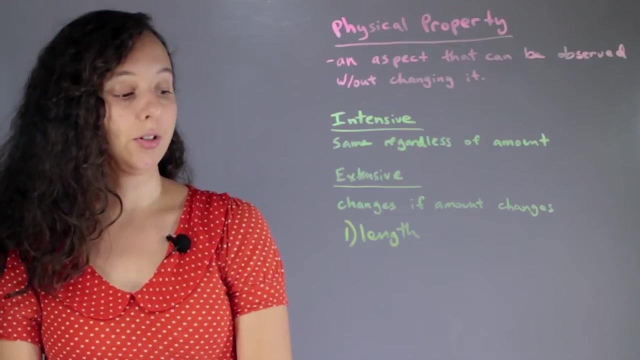 a match on fire, you can see what color it burns as, but you can only see that by changing the structure of the match. Okay, so let's review a little bit more about the structure of a match A little bit more. Intensive physical properties are same regardless of the amount, So a good 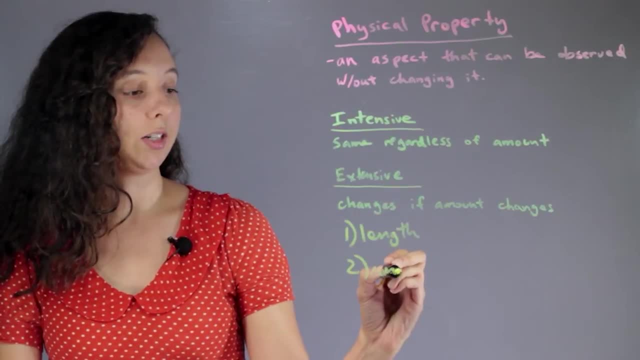 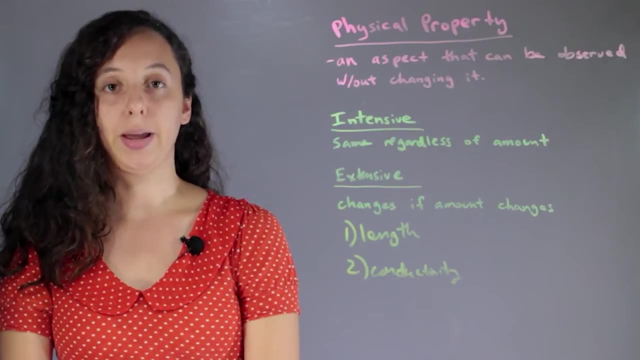 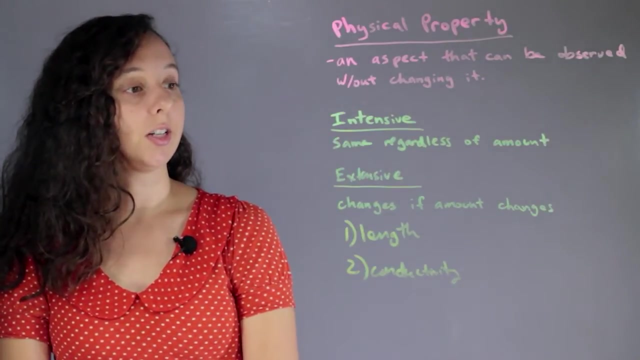 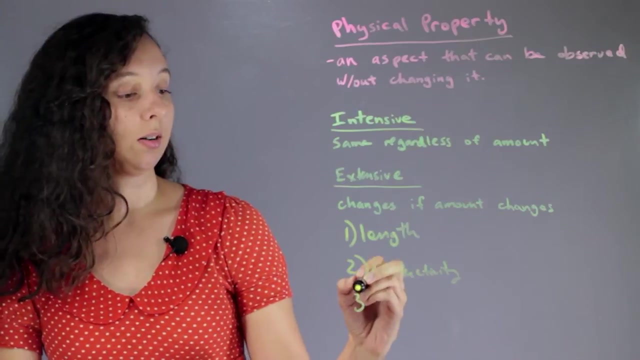 example of this would be conductivity. If you have a short wire or a long wire made of silver or gold, it'll conduct exactly the same. It doesn't matter Versus extensive changes if the amount changes. So this would be a good one for mass. If you have one pound of bricks, that's a lot. 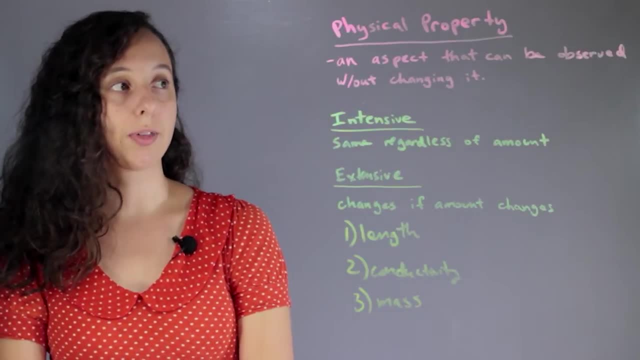 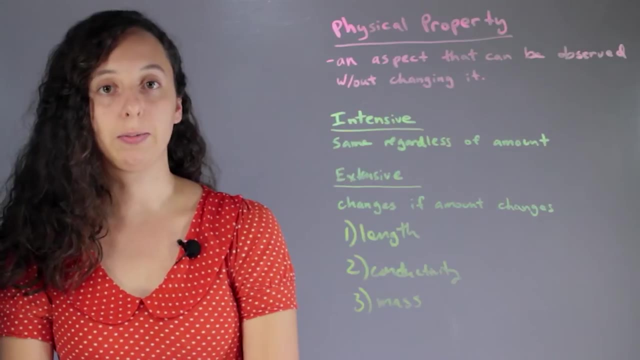 different than two pounds of bricks. You can observe both without changing it, So they're physical properties. But it changes if the amount changes, So it's extensive. These are the two types of physical properties, So without stringing along anymore, I'll give. 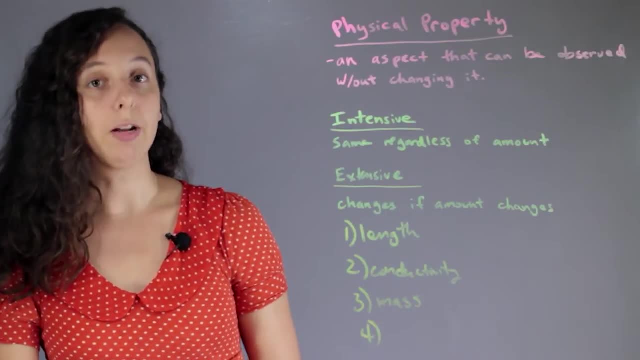 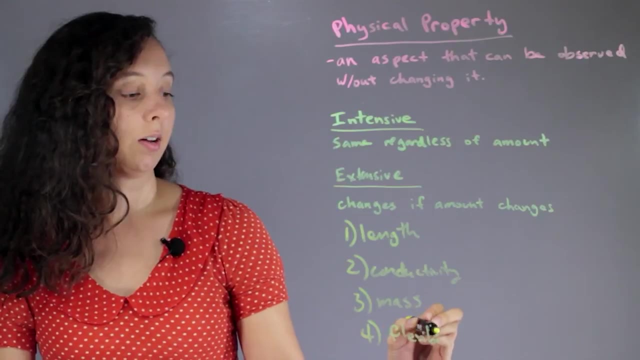 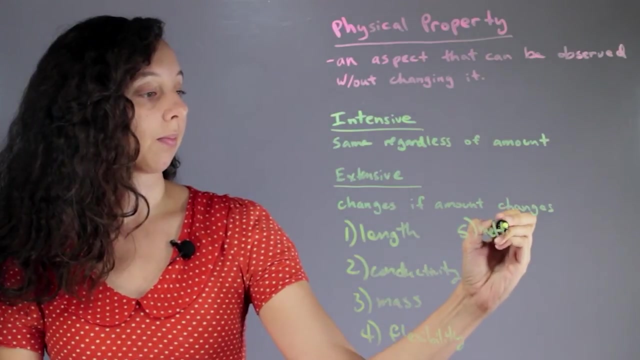 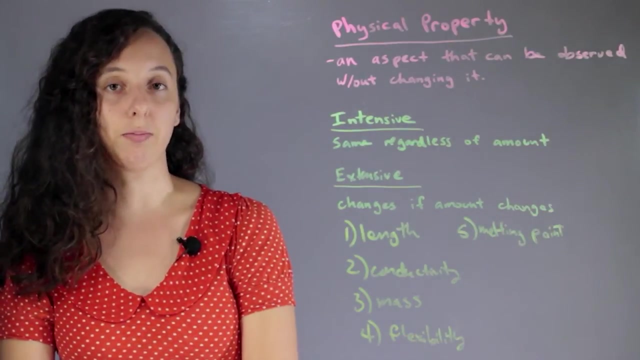 you the other seven, And of course there are many, many more. These are just an example of 10.. So we have flexibility, Don't have to do any chemical changes, Melting point, And so this is a good one to remember that, even though we're melting something to figure out the 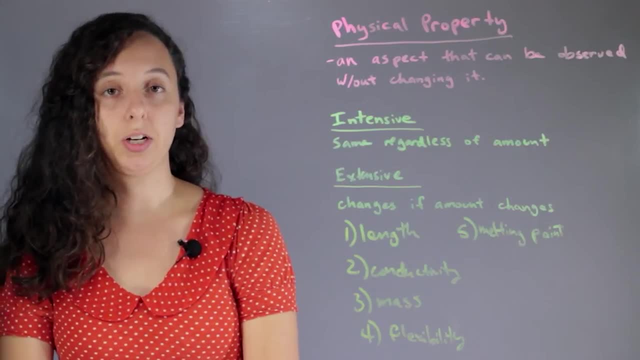 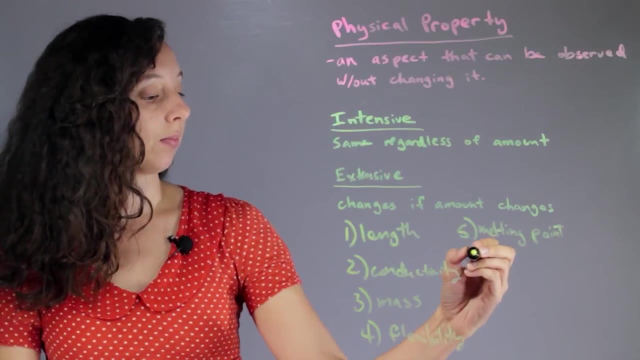 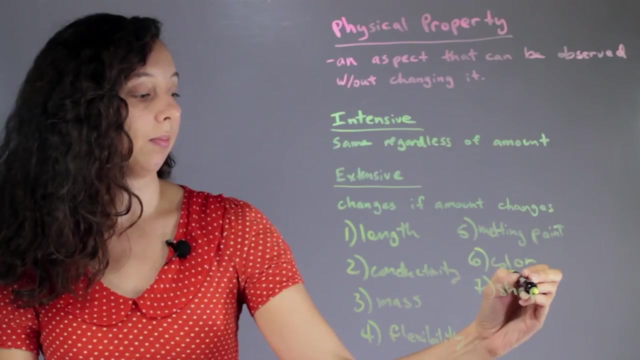 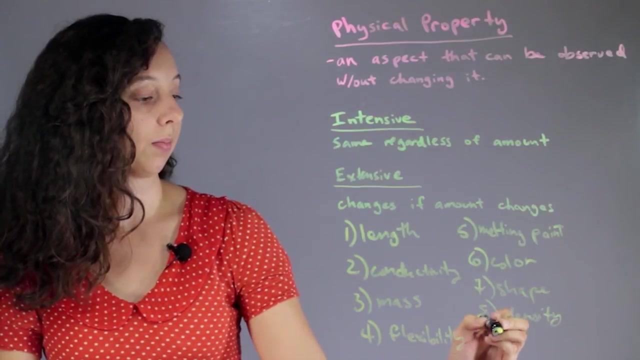 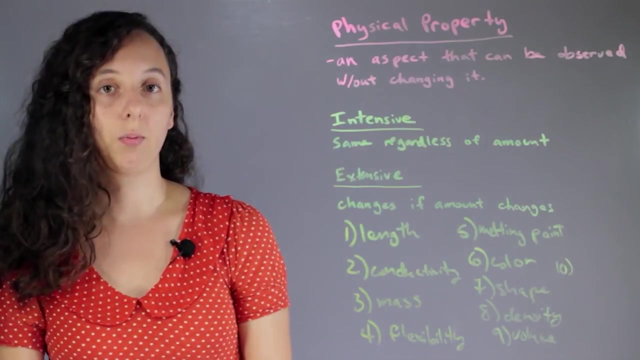 melting point. that's just a physical change, It's not a chemical change. So when you melt an ice cube, it's still water. It hasn't changed chemically. Color, Shape, Density, Volume And for number 10, one of the weirdest ones- luster. 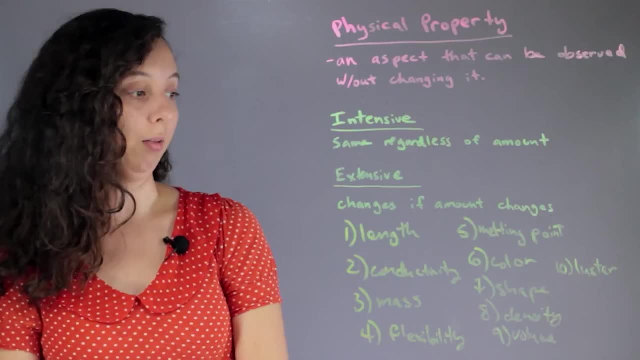 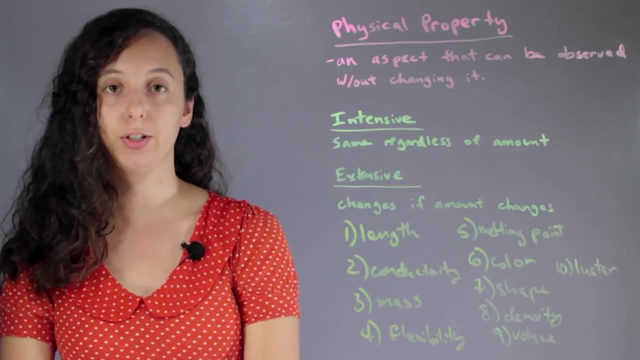 Which is just how shiny something is, but I just think luster is a weird word. All right, I'm Robin Higgins, and this has been 10 Examples of Physical Properties in Chemistry.